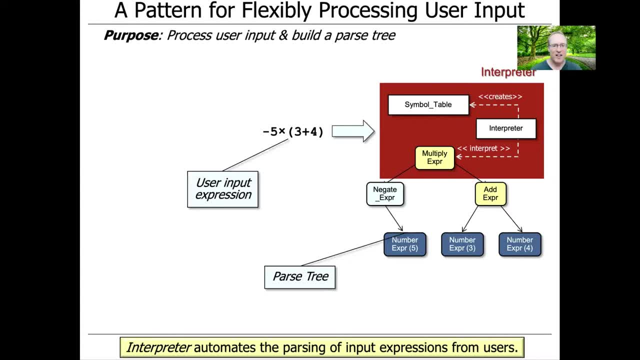 So keep in mind. what's going to happen here is that the user will provide their input either from the command line or from some kind of graphical user interface, And the interpreter will then use this input, which comes in as a string, to build a parse tree which is a representation of the information that's defined by the user in the input expression. 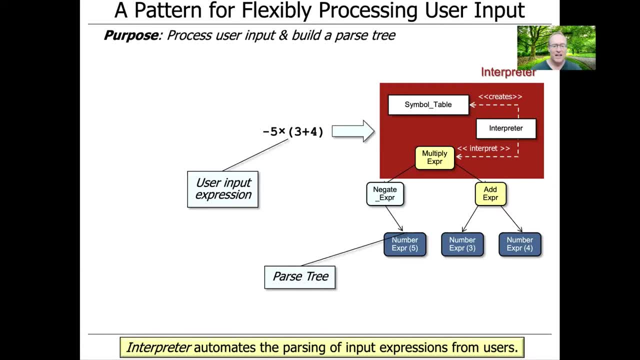 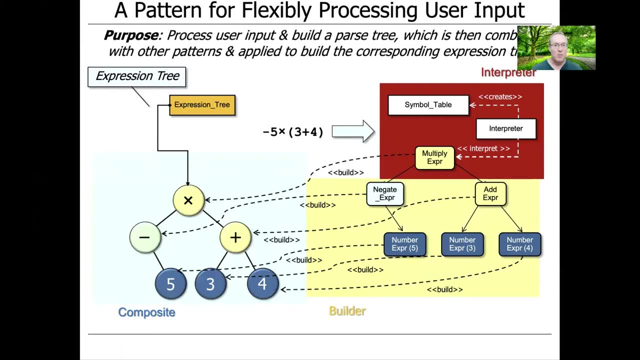 So we're going to apply the interpreter pattern to automate the parsing of the input expressions given by users, And then we're going to combine the interpreter pattern with some other patterns, Most notably the builder pattern, in order to be able to convert the parse tree representation into our composite expression tree. 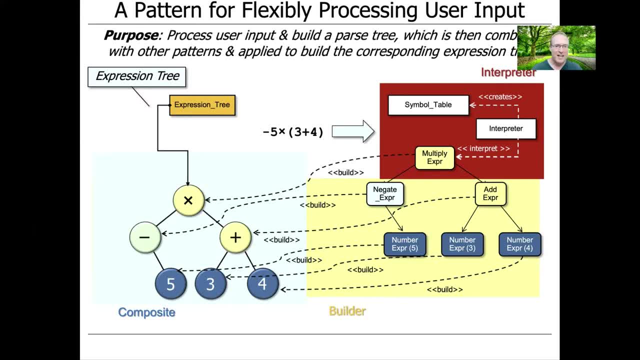 If you recall from our earlier discussion, the expression tree is a composite using the composite pattern and that will ultimately be provided to the user application code in the form of the bridge patterns abstraction, which encapsulates all the low level details of how the composite is actually structured internally. 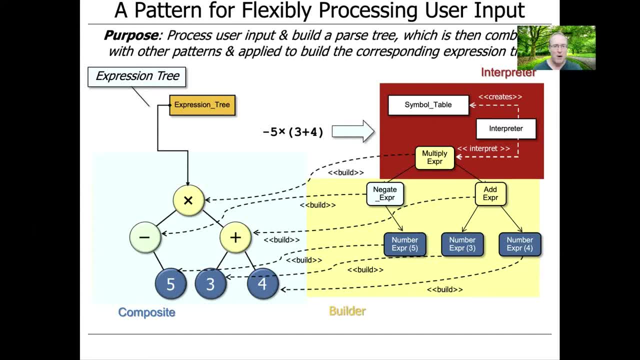 So you can see just from this diagram that there's multiple different patterns involved. We've got Interpreter and builder which will create the composite, and then that gets attached to the abstraction from the bridge pattern. Now the expression tree processing app can get its input from various sources. 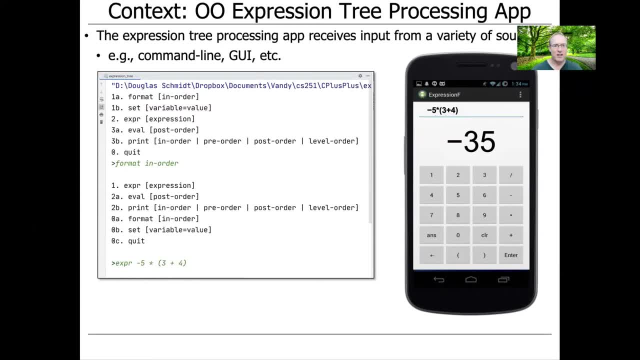 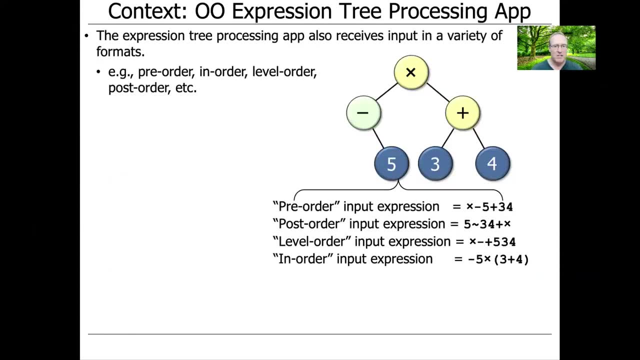 I mentioned that before. It can get it from the command line. It can get it from a graphical user interface, such as an Android app or some other app, And you also need to be aware that the expression tree processing app can receive its input in a variety of formats. 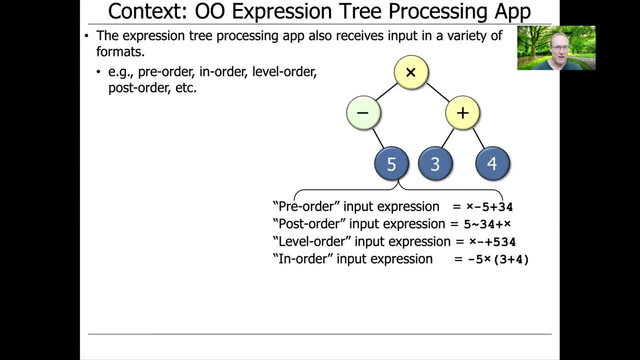 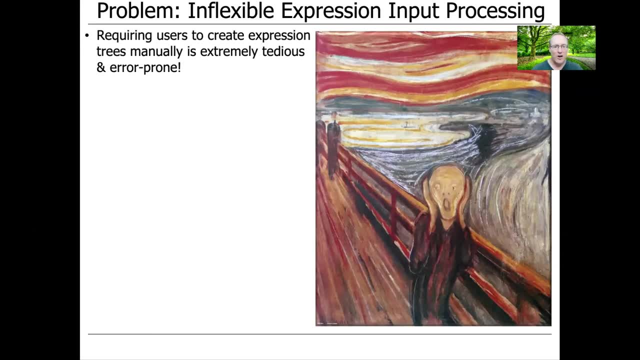 It can receive it in in-order format, level order format, pre-order format, post-order format, And so on and so forth, And what we don't want to do is require users to have to tediously enter all the input expressions manually. 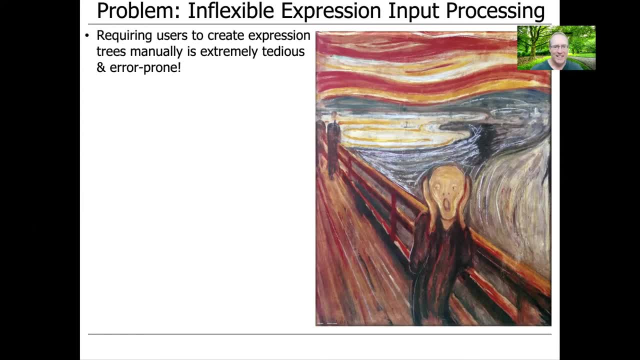 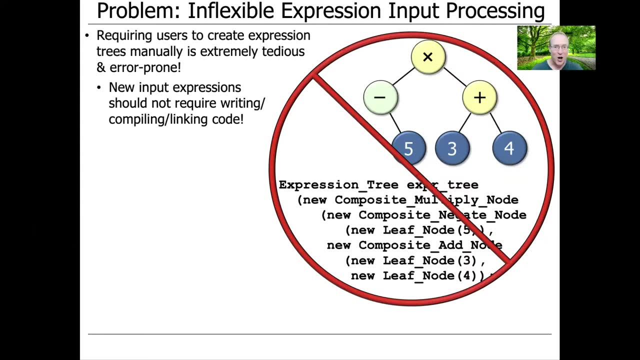 This would be unbelievably error prone and very, very tedious to do So. in particular, we don't want people to have to type input expressions by writing code and compiling code and linking code. That would just be monumentally bad. Likewise, we'd like to make it so that when users 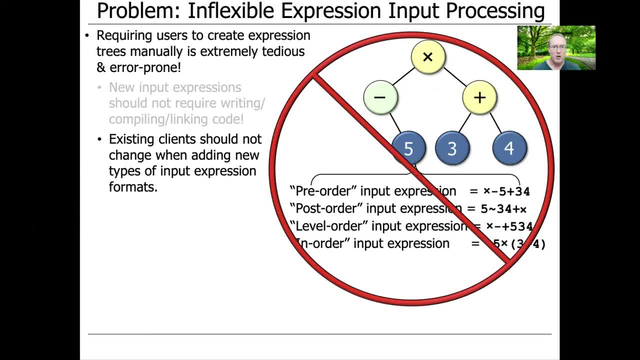 Come up with different ways of adding input, expressions, formats. Let's say they come up with yet a different way to do it. We really would like to not have to change anything about the existing code, And we'd like to also not have to change the structure of the program. 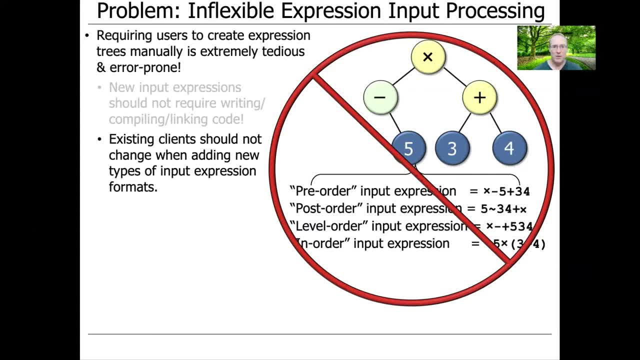 So in many ways this is very similar to the ideas we had when we were doing the composite pattern, where we wanted to be able to make changes to the underlying algebraic expression, abstraction- without having to go in and perform a lot of surgery on the composite itself. 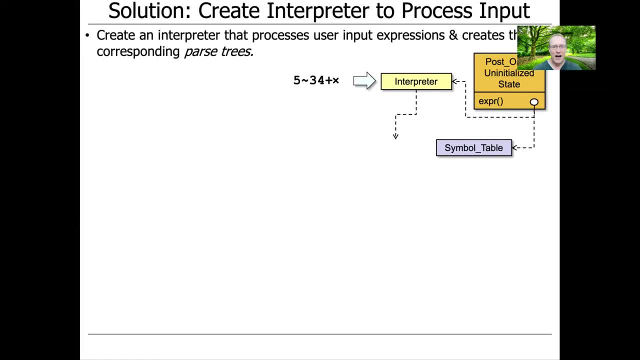 So how are we going to do this? Well, of course, we're going to apply a pattern. What pattern are we going to apply? We're going to be applying the interpreter pattern And we're going to use this to process the user input expressions and then create the corresponding parse trees. 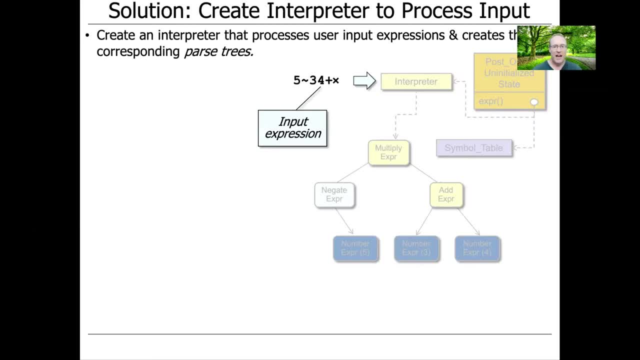 So you can see that we have an input expression like five minus three, four plus times, which is obviously coming in post-order format And that will then be processed by the interpreter And that will go ahead and create The corresponding parse tree. 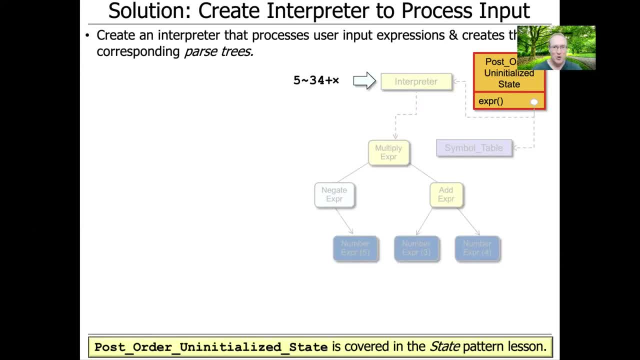 Now we're going to talk more about how this actually gets invoked later, when we talk about the state pattern, And we're going to talk about something called the post-order uninitialized state subclass, And that's where all the magic actually happens under the hood, to invoke the processing of the interpreter: 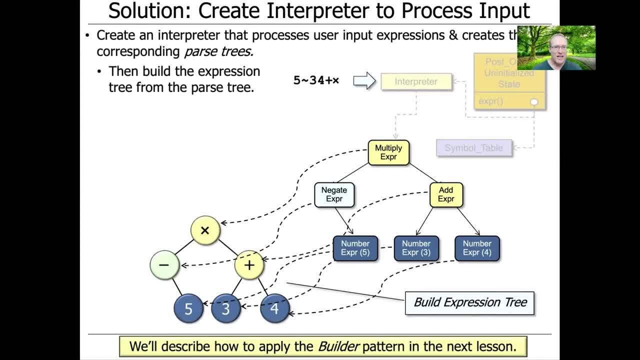 But that'll come a little bit later. Once we've got ourselves a parse tree that corresponds to the expression that was added or given by the user, we then are going to traverse that Parse tree And we're going to go ahead and build an expression tree. 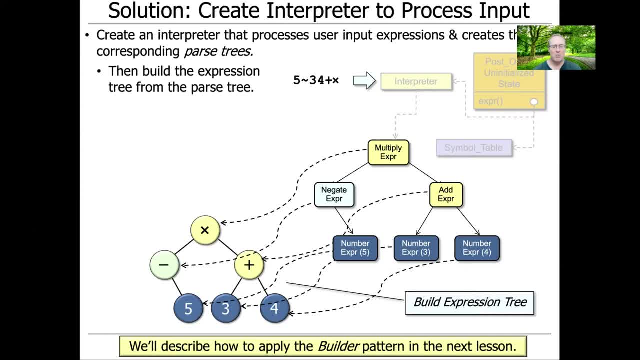 And surprise, surprise, we're going to apply another pattern here, And of course that's going to be the builder pattern. So we'll talk about the builder pattern in the subsequent lesson. Be aware that interpreter and builder are often used together in what's called a pattern compound. 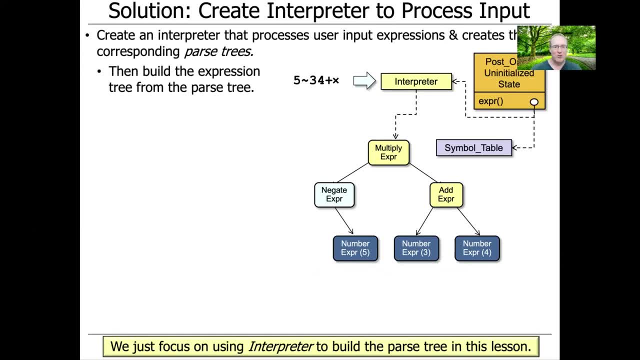 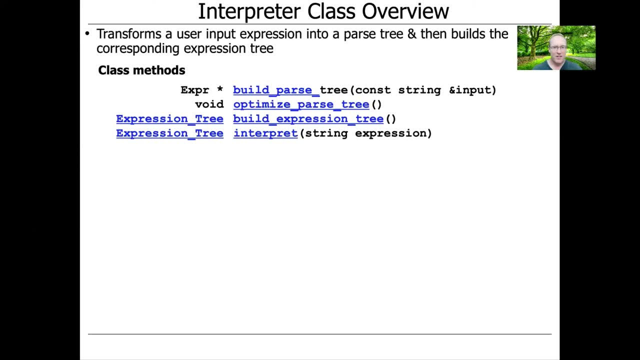 We're just going to focus on interpreter now, however, and we'll come back and talk about builder in the next lesson. So here's how we're going to define the actual interpreter itself. It's going to be a class, and the class is going to end up using the bridge pattern.